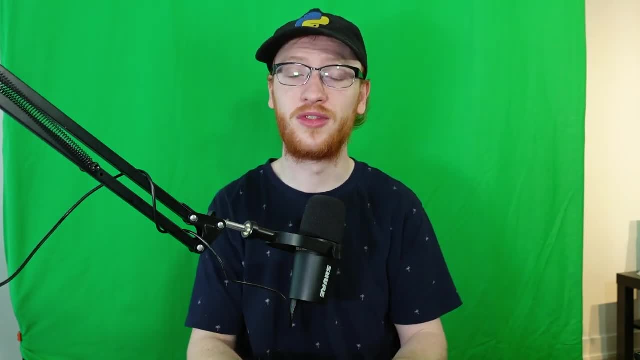 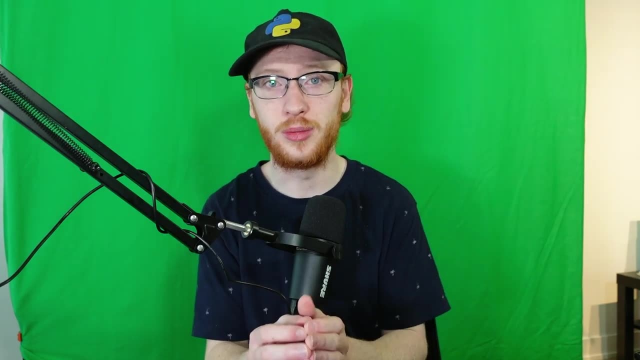 avoid the automation of chat gpt. we'll talk about that at the end. but firstly, you know data science jobs. they're there. however, exploratory data analysis is not quite what it used to be. it's a lot easier to actually get this stuff done. i think it's still very important to be able to understand python code to be able 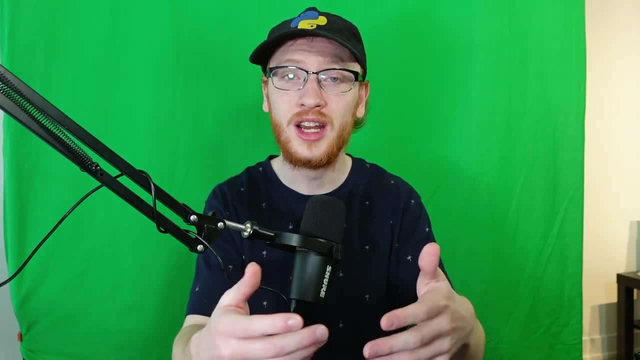 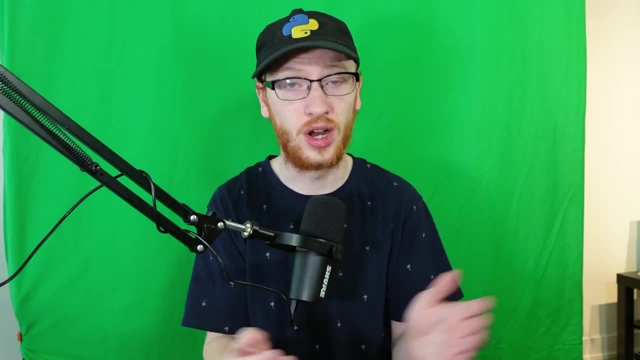 to understand the libraries so that you're able to do things and tweak the chat gpt responses as you need to. so it's extremely important to do these things because everybody's going to be able to code now. it's not as hard as it used to be. however, if you know the skills, you are going to. 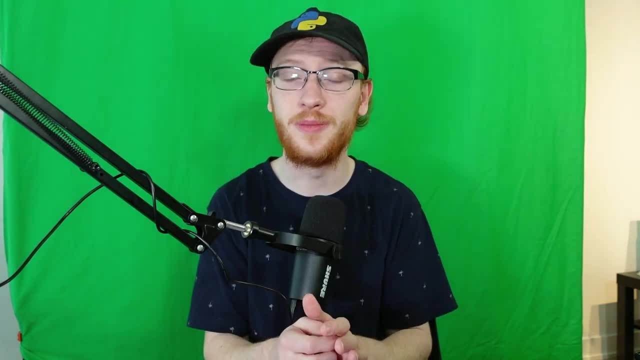 be much better than the people you're going to be able to work with, and you're going to be able to do some really broad logan dean's work for you, and you can do some pela noodles too, maybe faced security completely automatic. you can do a lot more stuff that people don't do and you can do. 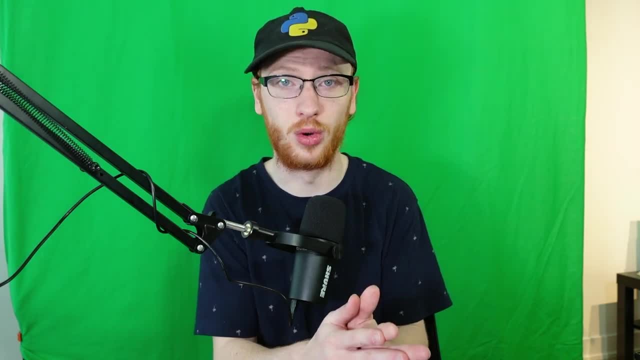 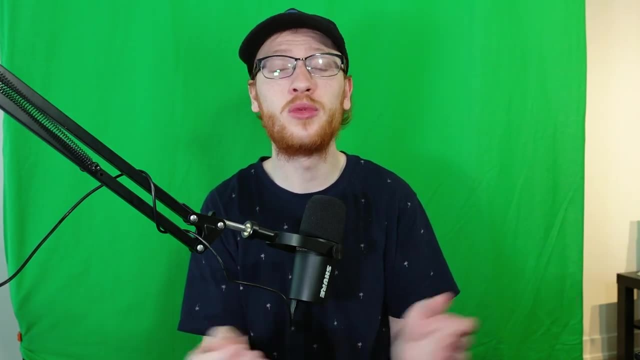 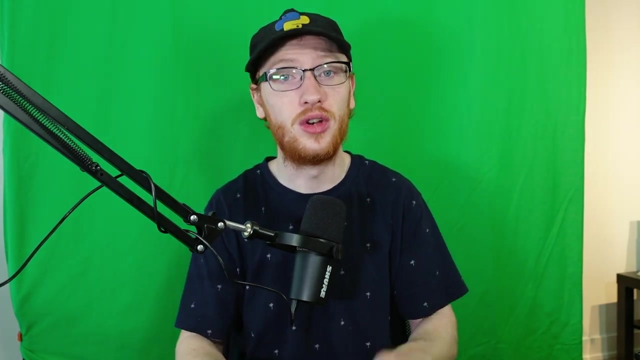 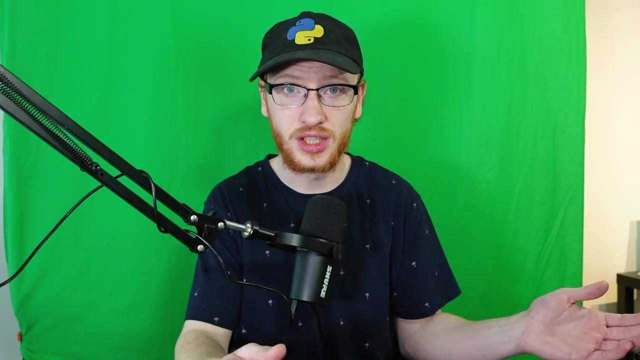 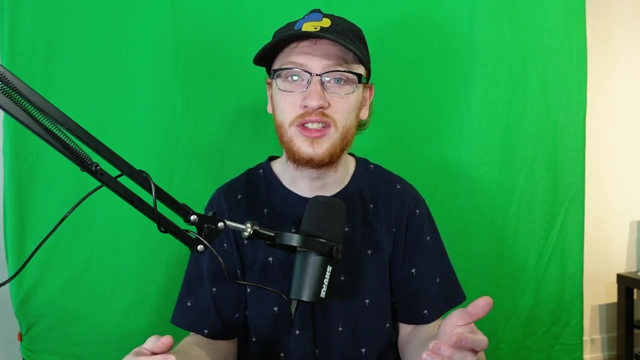 everything on your own. does that mean that there's page use? building your code open tells you stuff is going to be easier to make. so stay with this gpt education or somewhere and then come back and build projects, because anyone could build projects now like it's so easy. before what you had to do was to just grab a blog and then fiddle with it. 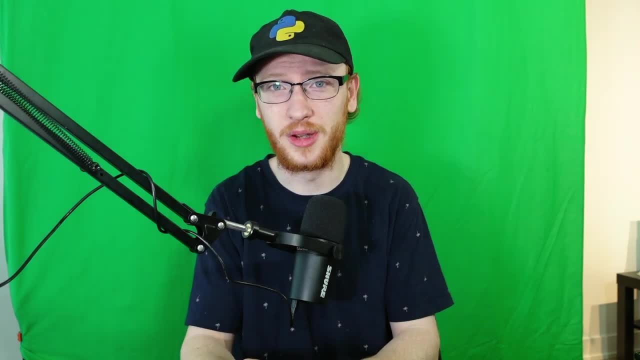 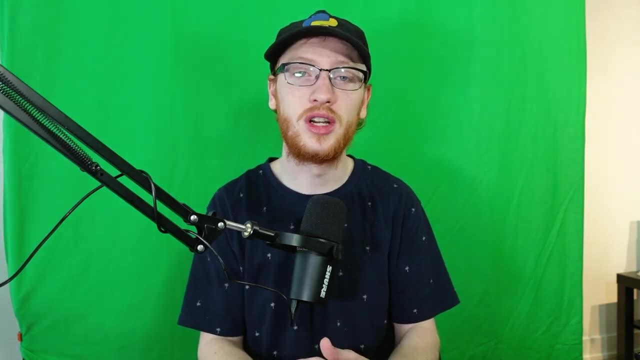 and then you'd probably get an error and then you'd fight with it. i know you've done this okay, so oftentimes we give up from that. jgbt is making it a lot easier just to build these projects online, and so you're gonna need to have all the skills: the software architecture skills, the of. 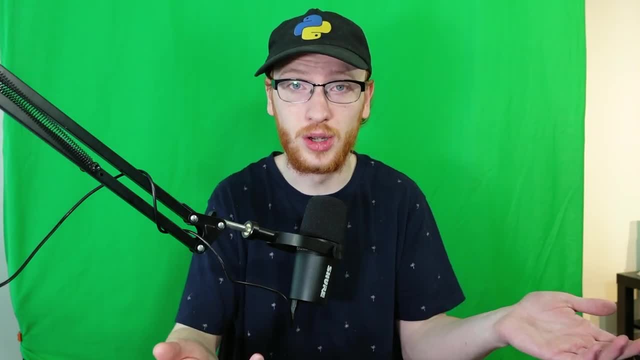 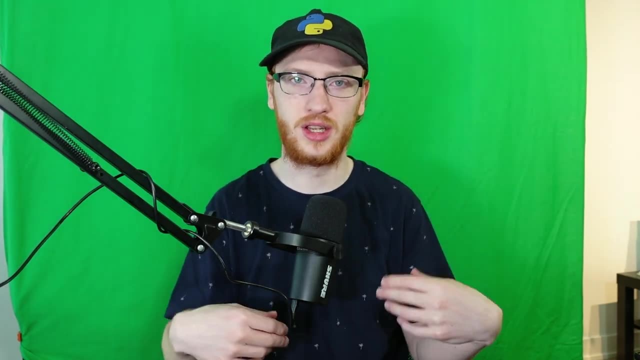 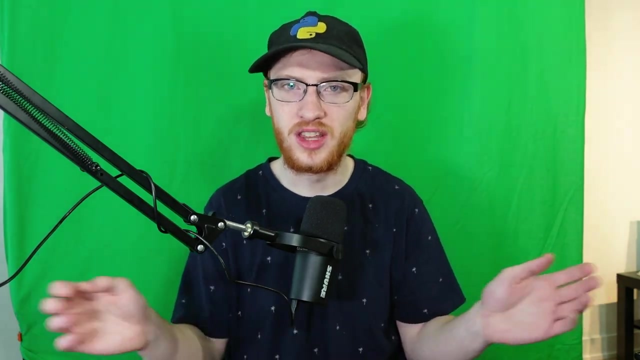 course, the, the libraries and the frameworks and the actual language itself, but more about building full applications. chat gbt is great at building code. it can. you can iterate with it and build applications very, very quickly. however, what it cannot do is piece things together. okay, it can. 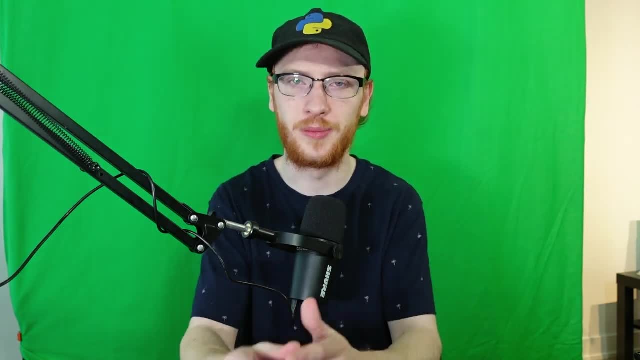 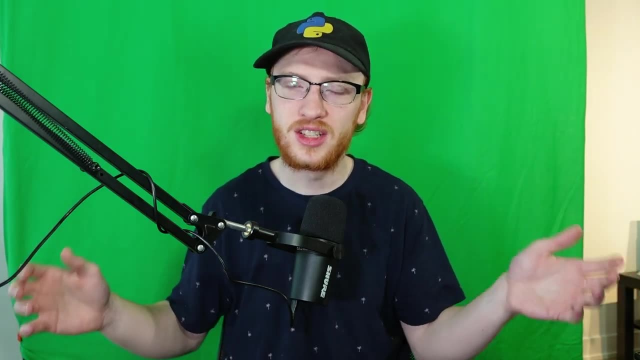 build individual lego blocks, but it cannot build a lego castle. you need someone- or companies are going to need people- that understand all of the lego blocks, what each of them do, and how to build a lego castle and how to build a lego castle. and how to build a lego castle. 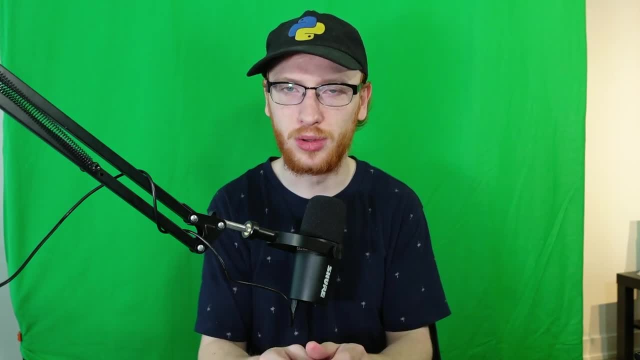 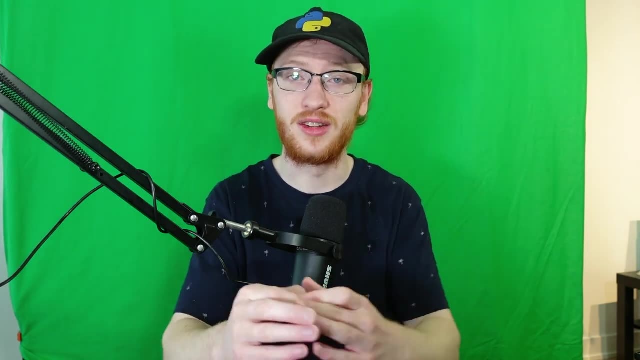 put them together. okay, it's going to be a lot more about actually putting things together and, of course, it's still writing code. i'm not saying that you're not going to need to write code, but it's getting faster and companies are going to need less people to actually write this. 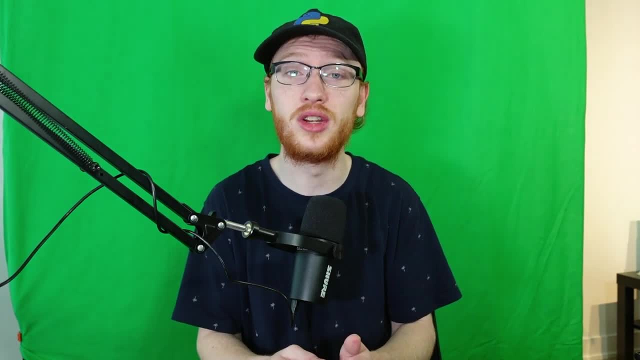 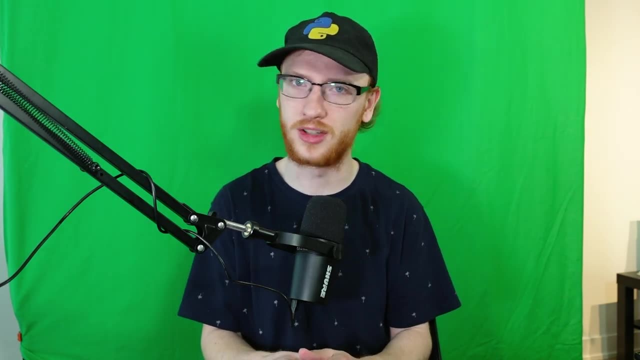 code because, like, developers are just writing code so much faster than they used to be. i'm working on a startup right now. you'll see the results hopefully this year- i really hope this year, hopefully by the end of the summer. but i am writing code extremely quickly right now in languages that. 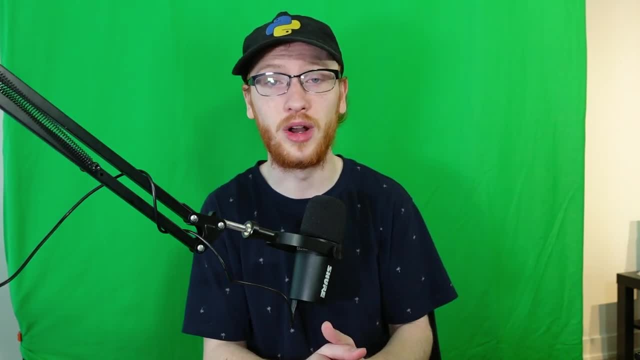 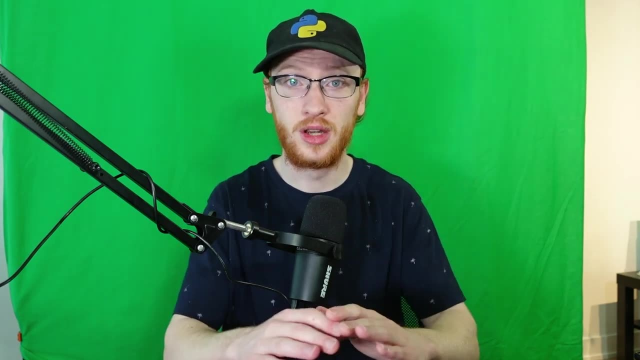 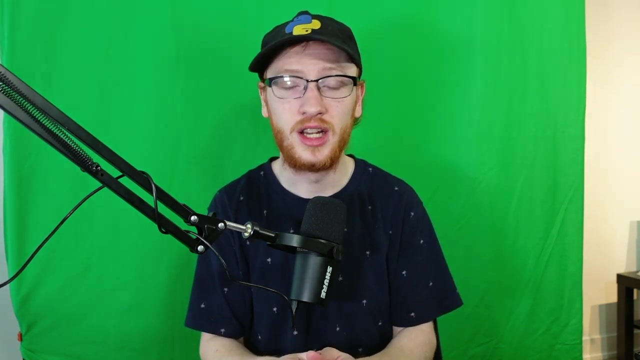 i am learning at the same time, like javascript. i don't know very well, but with chat gpt, i'm writing javascript code and i am using it all the time. so, trust me, coding is just easier than it used to be, my god. but anyways, chat gpt is so so good at writing code in many areas, and so it's going to. 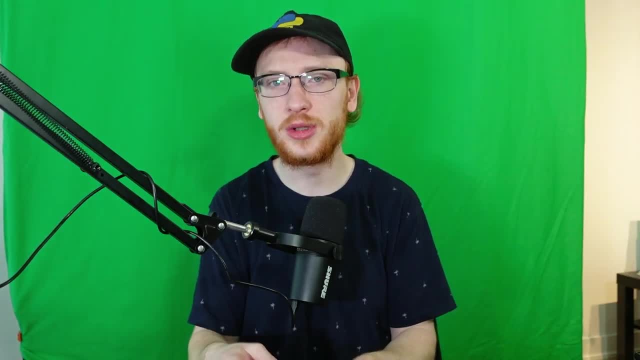 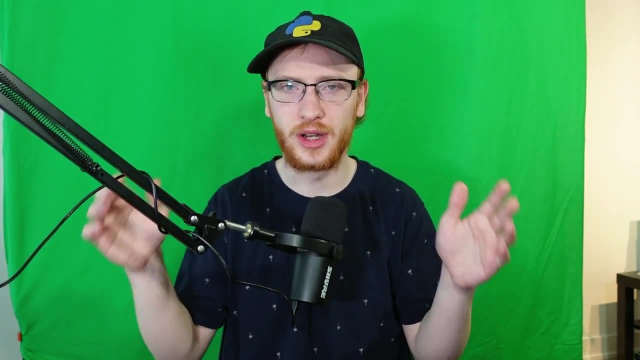 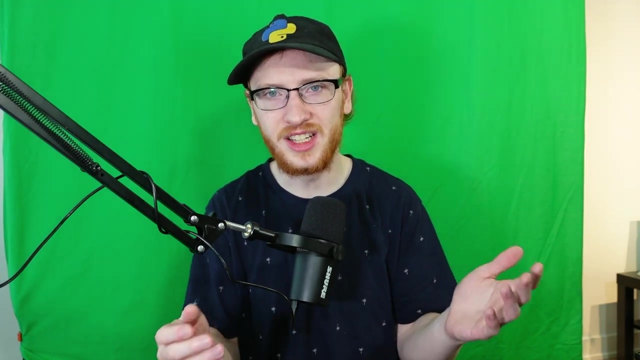 be a lot more about knowing these individual lego pieces, being able to put them together, and 100- this is what you absolutely need to know- is gcp aws, azure, building virtual applications, putting all the pieces together to build a final product. because, again, data analysts, data exploratory, data analysis, simple data science stuff, it's still useful. 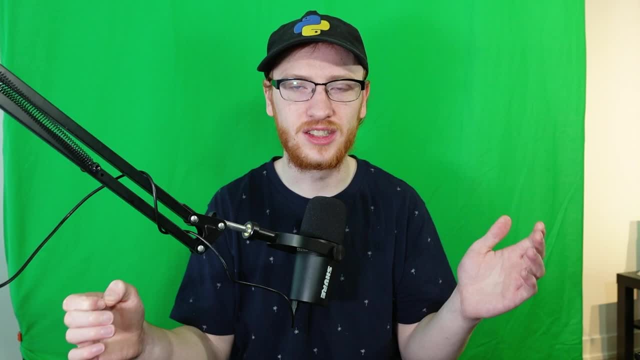 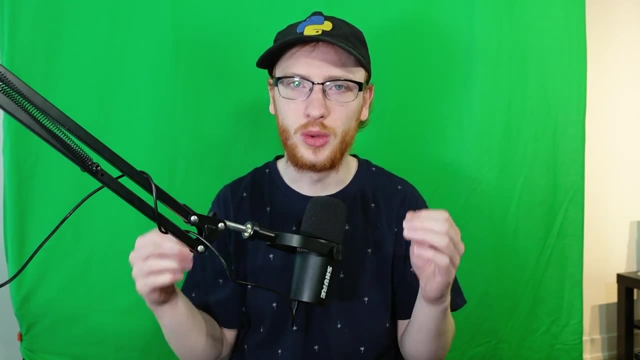 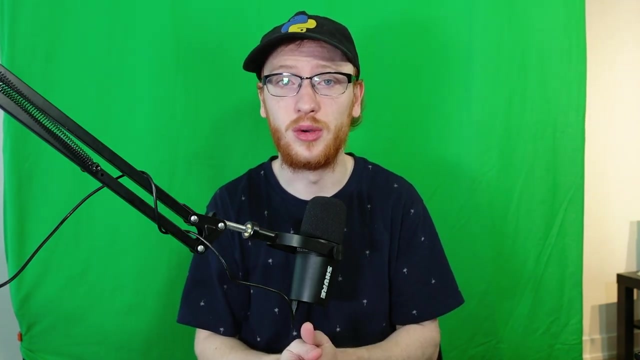 it's still extremely useful, and i'm not saying that it's going away, however. it's just easier. you're still going to need to know all of these skills. if you're a data scientist, you absolutely should still know python, all these visualization libraries, sql, all the normal stuff like tensorflow. 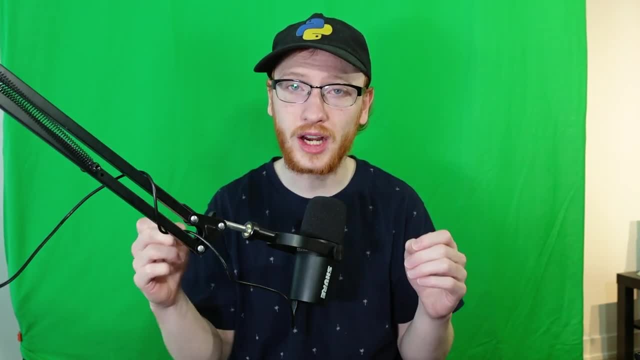 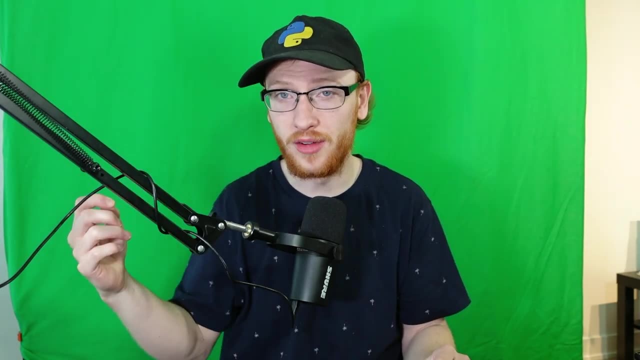 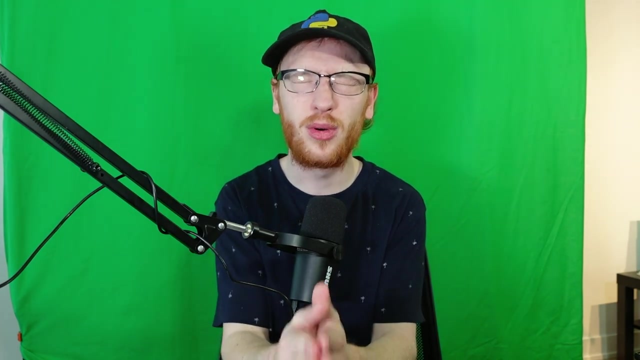 pytorch, whatever for machine learning models. however, your actual job is getting easier in some ways with the. you know traditional analytics is getting easier. however, it's going to merge into building full applications. okay, i've said this in previous videos: it is more important than ever right now to learn all of this data science stuff. 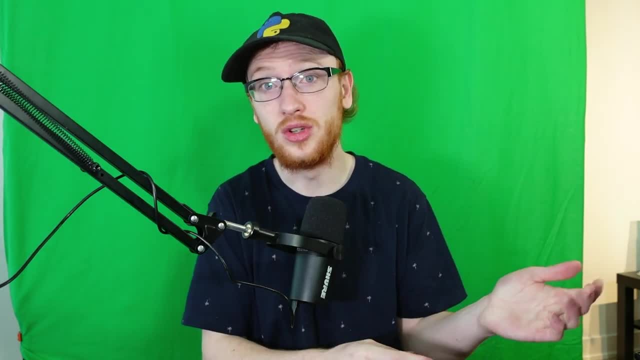 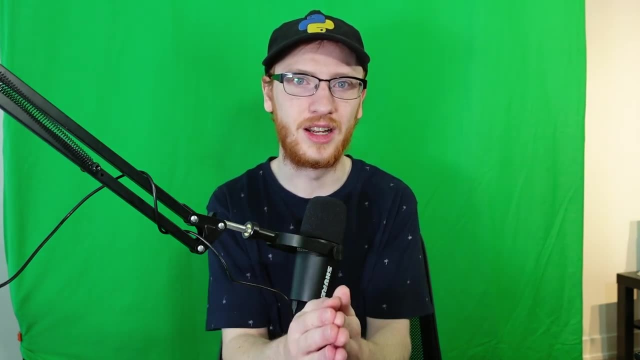 and then learn how to build actual applications. and you can do it in the reverse way if you want. you can absolutely build applications and then you can learn data science. there's still going to be a lot of roles in data science. however, it's going to be a lot of roles in data science. 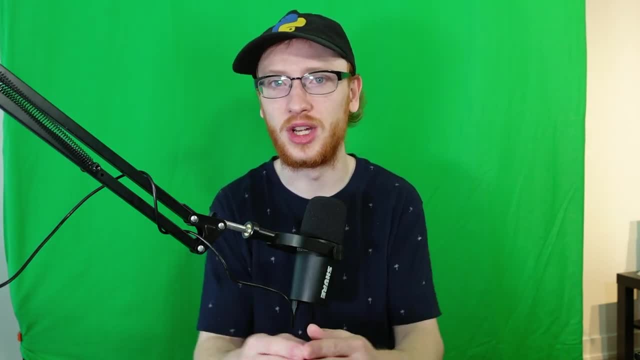 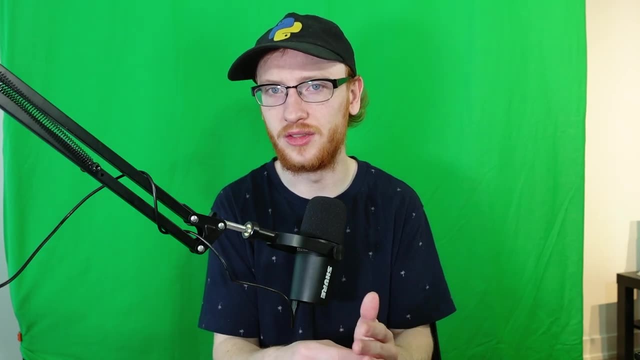 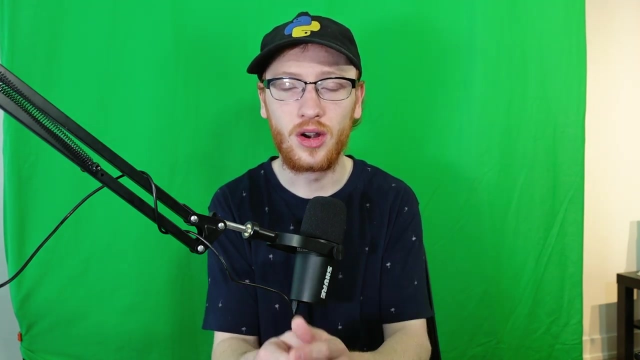 where they're merging into doing multiple things at the same time, using your analytics to build these applications. okay, now there's still going to be those base analytics roles where you're just doing simple visualizations and stuff and presenting them. however, it's hard to say how.